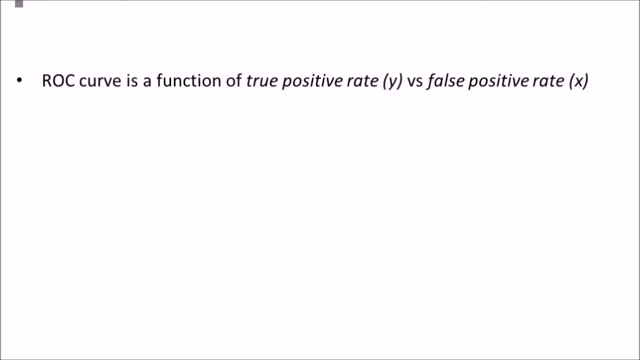 true positive rate on the y-axis and the false positive rate on the x-axis. So this is what an empty ROC curve looks like, which has false positive rate on the x-axis and the true positive rate on the y-axis. So now true positive rate. it is also known as sensitivity, and which is also. 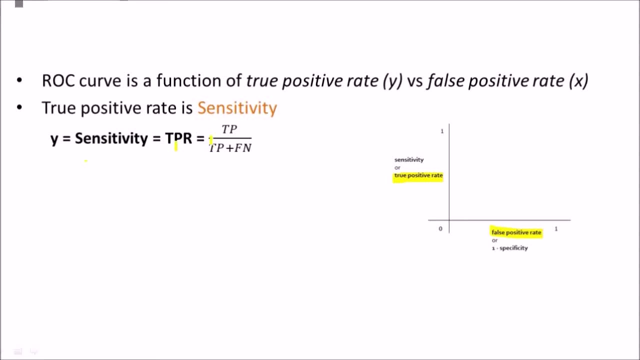 known as recall Y on the y-axis. as I said, it is sensitivity and the formula is true positives upon true positives plus false negatives. Just basically trying to tell us, out of all the real positive samples in the data, how many did I? 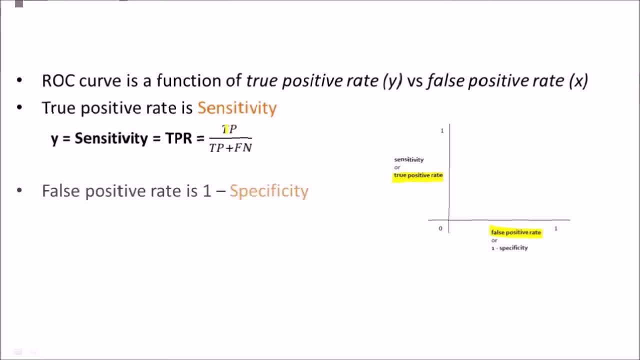 correctly predict to be positive. So this is sensitivity and false positive rate. It is 1 minus specificity, where specificity is equal to true negatives upon true negatives plus false positives, And specificity is trying to tell us that, out of all the times that the real class 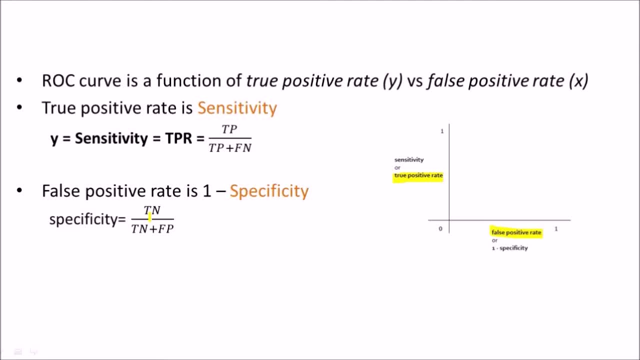 was negative. how many times did I correctly predict the class to be negative? So 1 minus specificity is the false positive rate and it is false positives divided by true negative plus false positive. So now false positive rate is telling me that, out of all the 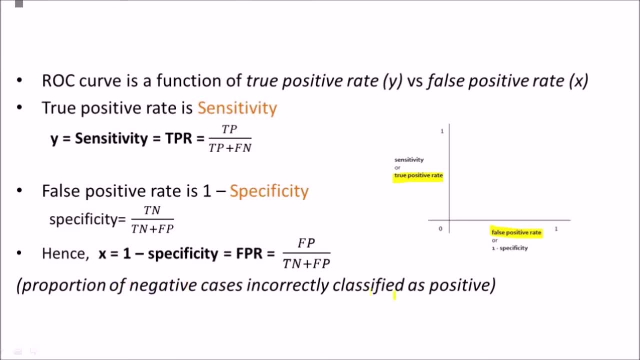 negative cases in the data. how many did I incorrectly classify to be positive? So, for example, there were 100 negative cases in the dataset and if I predicted to哥isi phi of them to be of the positive class, then my false positive rate would be ϕ upon. 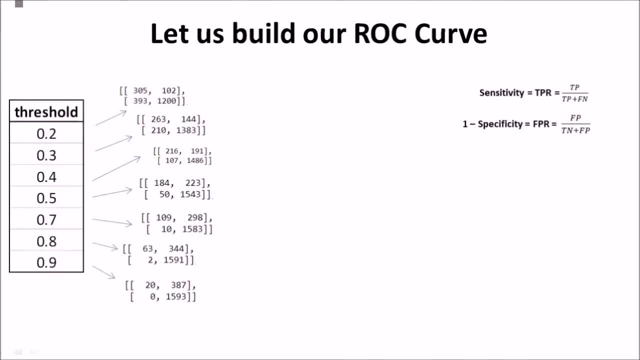 which is 5%. now let us build a ROC curve. now, as we talked earlier in the lecture on the precision recall curve, we saw that we can draw various confusion matrices by changing the threshold value. okay, so this is for the same classifier, but for different threshold values we can get. 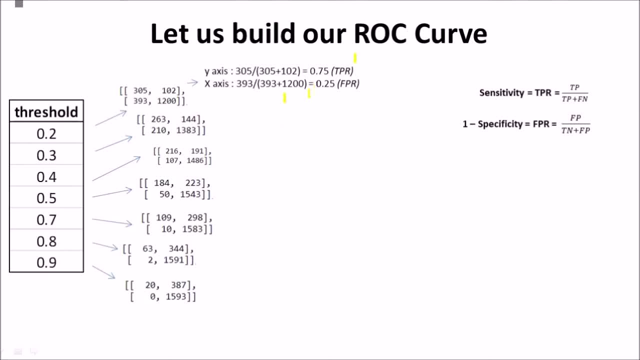 different confusion matrices and we can calculate the true positive rate on the y-axis and the false positive rate for the x-axis by the respective formula, as we see here. okay, so for each confusion matrices we can calculate these metrics and for the first point we get this particular point. 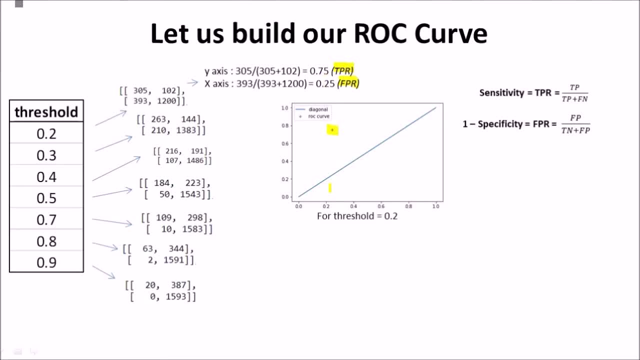 at 0.75 on the y-axis and 0.25 on the x-axis. okay, and similarly for all of these threshold values. when we draw the points, when we calculate the y and x-axis points, we get this kind of a curve. and for 30 equally spaced threshold values between 0 and 1, i get this kind of a curve. and this is my. 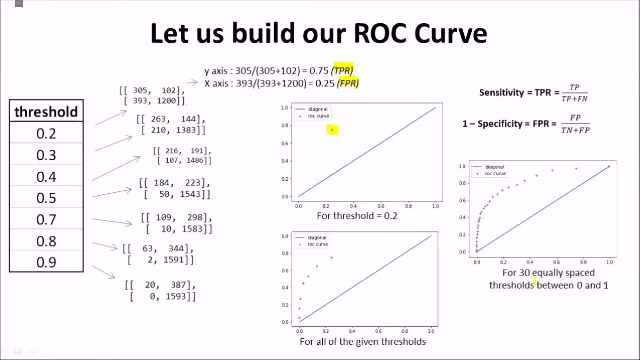 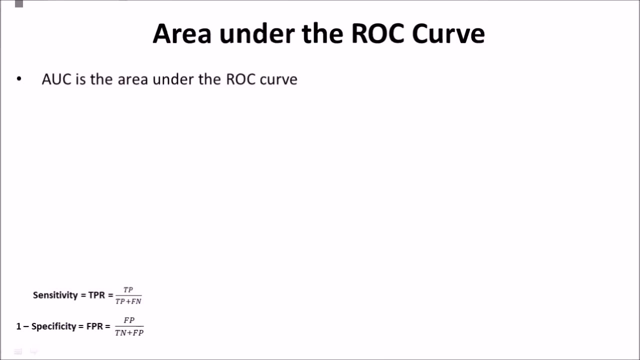 ROC curve. basically now, internally the, the selection of threshold value, is not equally spaced. but just take it for granted that if i take these 30 threshold values i get, i'll get this kind of a curve. okay, now, what is area under the curve? well, area under the curve is basically the area under the ROC curve. we know that the x-axis 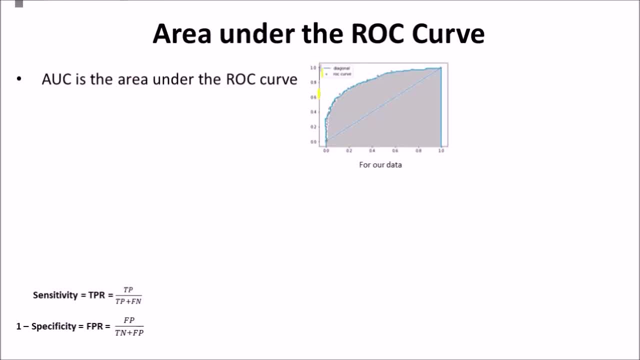 is going from 0 until 1 and y is also going from 0 until 1, so my area under the entire curve is 1 square unit. right, because it is a square of unit 1, so my maximum AUC can be 1 and for the perfect classifier, my AUC will be 1. okay, so this classifier will not make any. 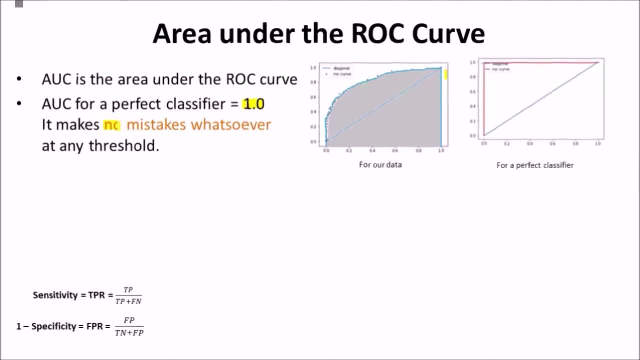 mistake whatsoever at any given threshold. so my perfect classifier would look something like this: okay, so my perfect classifier would touch this point, which is the point of 0 comma 1. so 0 means 0 for the false positive rate and 1 for the true positive rate. okay, so if my classifier looks like: 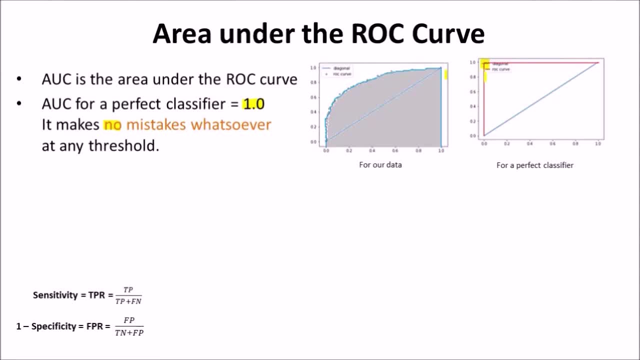 this. it is a perfect classifier, and the better my classifier, the closer will that be to the classifier, be to this red curve or basically to this point of 0 comma 1. so now you must be wondering: for what case will we have a perfect classifier? we'll just imagine that we have six. 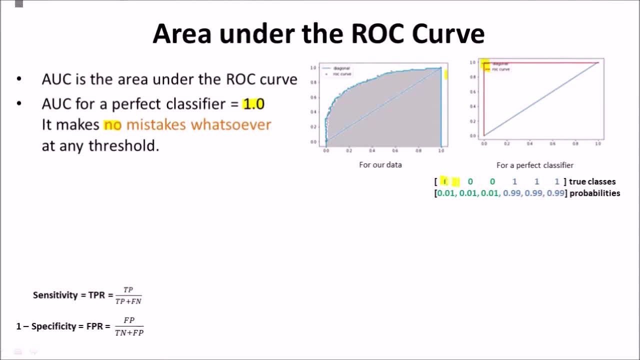 cases in the test set. out. of these, the first three people do not have the disease and the next three people have the disease. okay, so these are the true classes in the test set, and just assume that my classifier is so good that the predicted probabilities are 0.0. 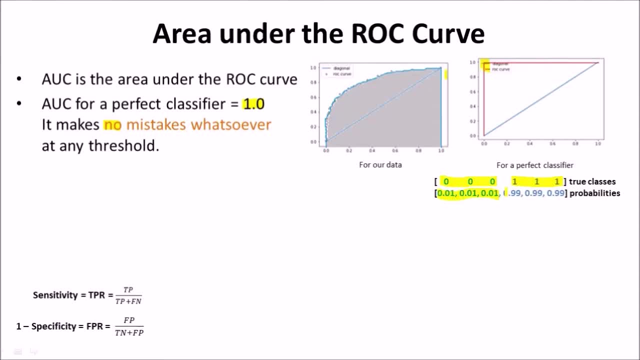 1 or 1 percent. for all of these three people and for the next three people, my classifier says that these people have 99 percent probability of having the disease. okay, so now if I draw confusion matrices for any particular threshold value between 0 and 1, I will get a perfect classifier. 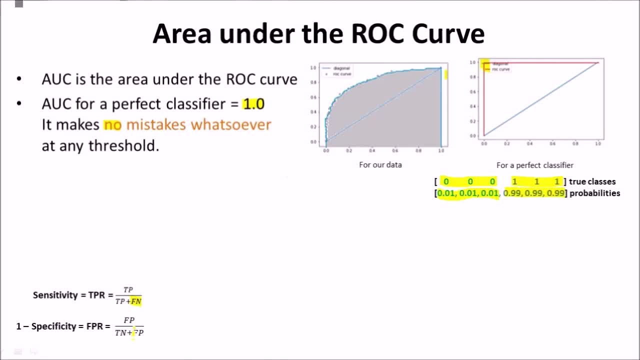 because now I will not have any number of false negatives or any number of false positives. so my sensitivity will be equal to 1 because true positive by true positive and my false positive will be equal to 0 because I have no false positives. so if my false positive rate is 0, then I'll have 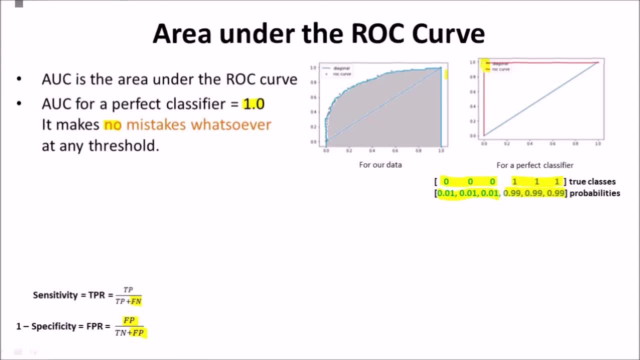 this particular point at 0 comma 1, so this is my perfect classifier. okay, so this is the basic understanding, although it is rarely the case that you have a perfect classifier, but just for demonstration purposes as to how it can be the case. so worst classifier will basically lie on. 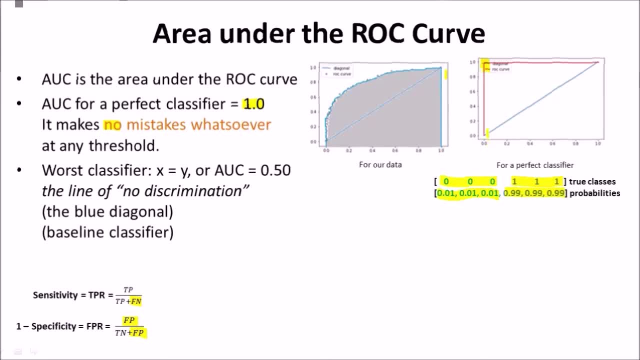 this particular diagonal line. okay, so this will basically mean that if I have a classifier that is on this blue diagonal line, it will have an area under the curve of 0.5 right, because this blue line is dividing the whole square into two parts. so this: 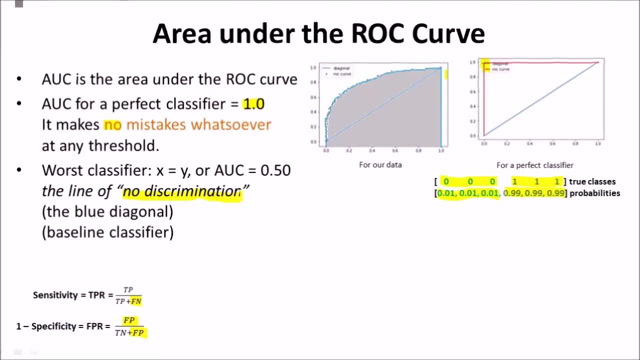 is also known as a line of no discrimination and hence it will have an area under the curve of 0.5. okay, and it is also known as a baseline classifier, that if you are trying to judge a classifier whether it is good or not, then you can check whether how close that classifier. 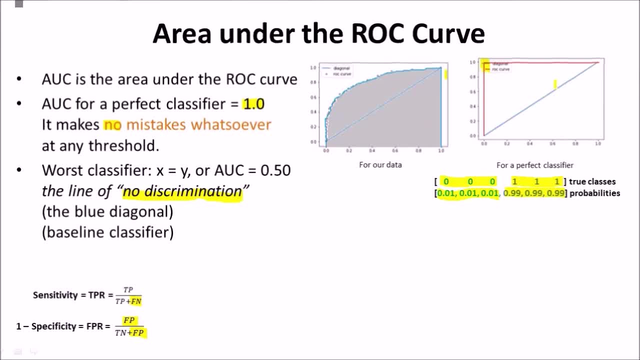 how close that area under the curve is to 0.5. if it is very close to 0.5, then it means that your classifier is not at all good. now, if I have two classifiers, for example, if a is my random forest classifier and b is my logistic regression classifier, then a has a higher area under 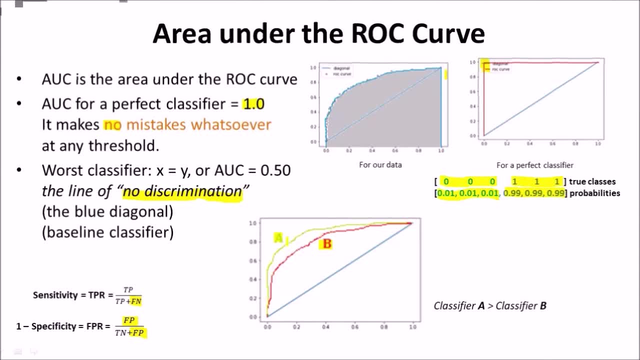 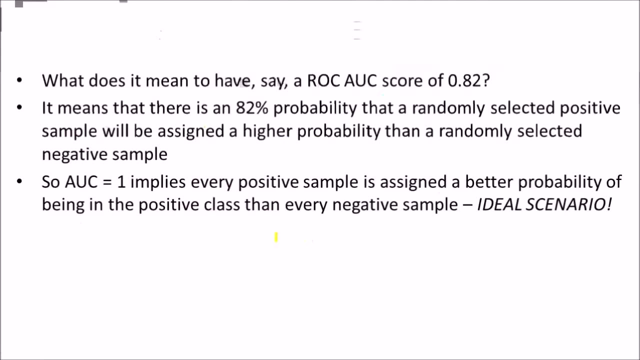 the curve than b, and hence my classifier a will be better than classifier b. and also, you see that this classifier a is closer to this point of 0 comma 1: the closer the ROC curve is, the better the classifier is. now you must be wondering what does it mean to have, say, a ROC? 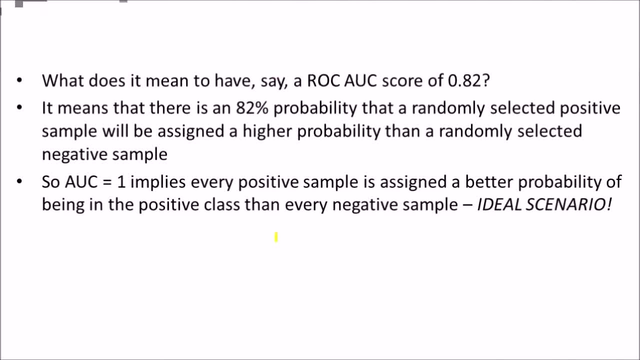 score of 0.82. so what does it really signify? well, it means that there is an 82 percent probability that a randomly selected positive sample will be assigned, a higher probability than a randomly selected negative sample. so if my ROC is equal to 1, so it implies that every positive sample 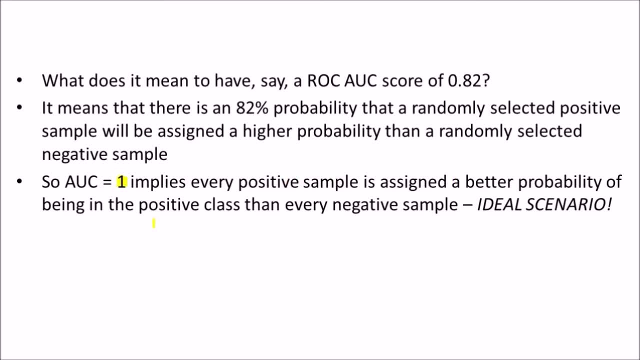 in the data set is going to be assigned a better probability of being in the positive class than a negative sample in the data set, which is obviously an ideal scenario. right, because that is what we want. we want the positive samples to have a higher probability than the negative samples of being in. 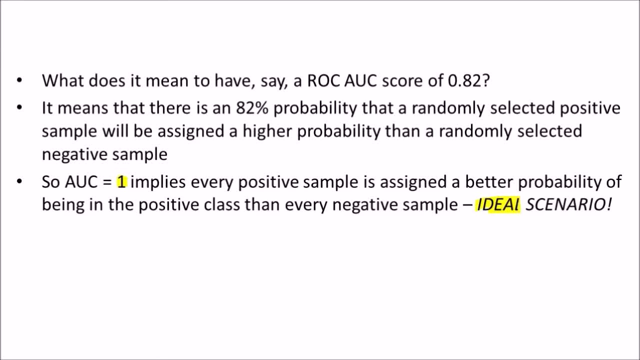 the positive class. that is what the area under the curve actually signifies. now, the better a model is, the farther away will a model be from this blue diagonal line. okay, so on this green side a model will be good, and on this red side a model will not be so good because it will have an area under the 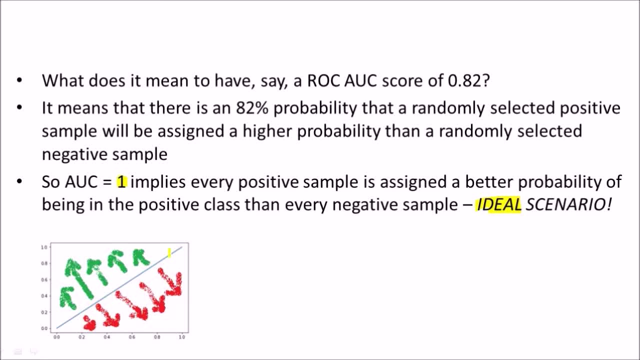 curve of less than 0.5, when we know that the baseline should be 0.5. now just a little pointer: if you have a classifier that has points on the other side of the diagonal line, so this basically what it means is that my classifier is just inverting the response of what it should be giving. so if it is saying that a 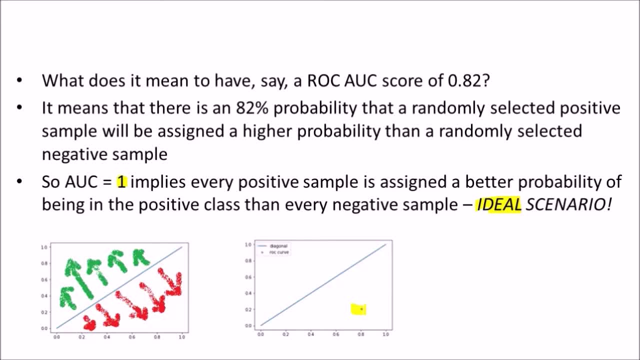 person belongs to the positive class, then actually it means that the person is belonging to the negative class. so what we can do is we can project this particular point exactly to this point here. okay, so we're just projecting it off this blue diagonal line. so now what it means is that for 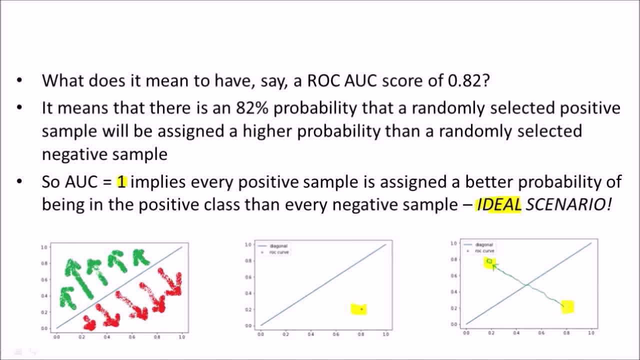 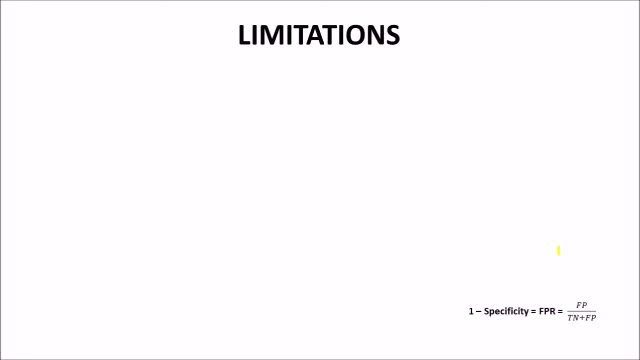 example, if a person was diagnosed to be positive in this case in this classifier, then actually he will be classified as negative in this classifier. okay, and suddenly a classifier is now good one because it has an area under the curve of greater than 0.5. now there are a few limitations of using. 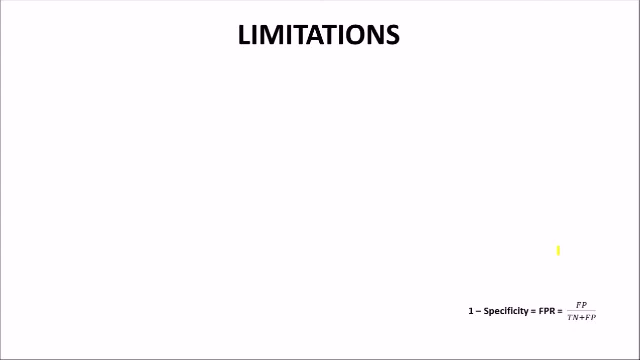 the rock AUC score and using the ROC curve in general. first is that the ROC curves should not be used when the number of negative samples outnumber the number of positive samples by a huge amount, or to say there's a severe class imbalance. the second one is the ROC curve should not be used when we are only concerned about prediction. 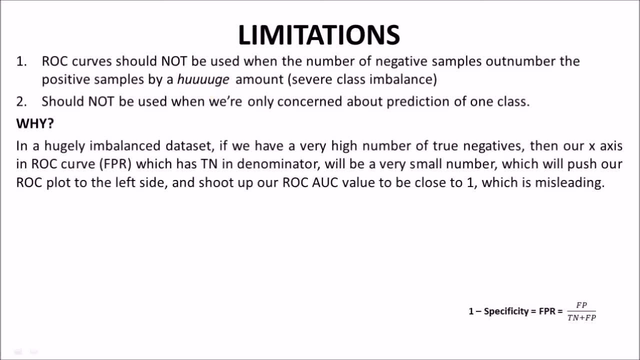 of one class. so why is that so well in a hugely imbalanced data set, if we have a very high number of true negatives? okay, so just imagine that if we have, for example, 10 positive samples and thousand negative samples, so we'll have a very high number of true negatives, right? 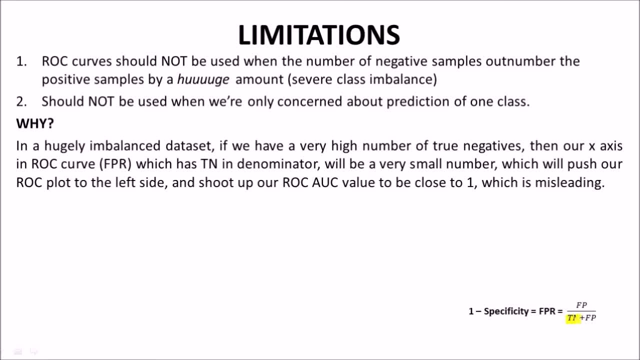 so, if we have a very high number of true negatives, if you look at this false positive rate formula, which is my x-axis, i'll find that my denominator will become very big number and hence my false positive rate will shrink to a very low number. so if that is the case, that a false positive rate